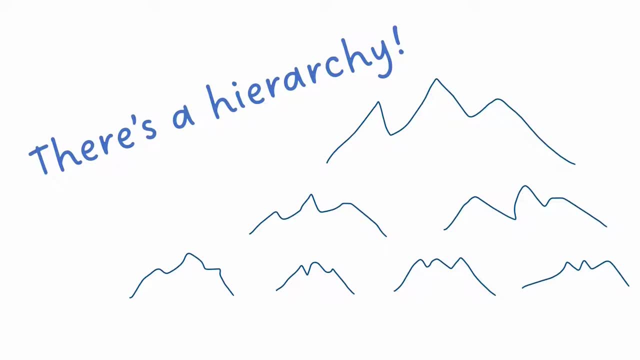 around and learn about this. So, starting with scale invariance. So imagine we have a curve and then, when we zoom in on this curve, we actually find that the curve isn't smooth. It has numerous little protrusions and you see more and more of these the closer you look. The classic example of 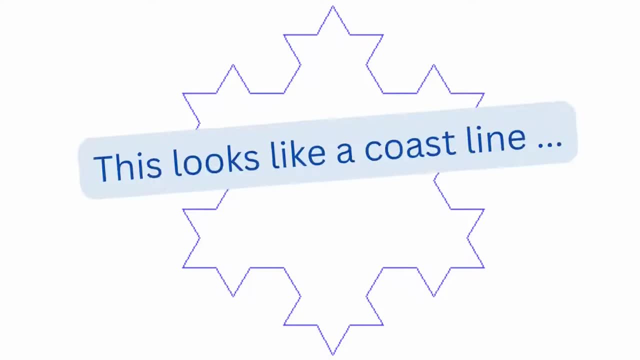 this is taking a map which is relatively coarsely shaped and then taking a map which is relatively drawn, but the further you zoom in on it, the more and more little bays and peninsulas that you see. Often it's the coast of Britain that's used for such an example, and I found this neat little. 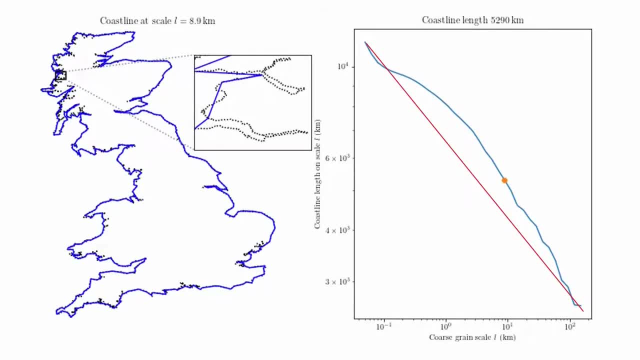 example here put out into the public domain. so I thought why not, let's have it here. But you can see here that the more detail you represent in mapping Britain, the longer its coast appears to be, And when you plot the length of the coastline is measured with different degrees of coarseness. 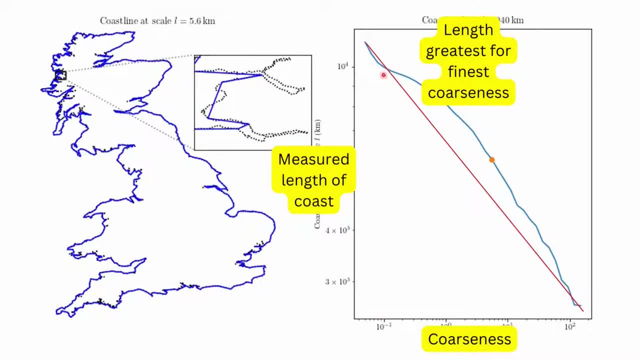 on a log log plot, like on the right, you get approximately a straight line, and the slope of that straight line is generally what people refer to as the fractal dimension for the particular object you're measuring. Now, it's really important to mention at this stage that the coast of Britain 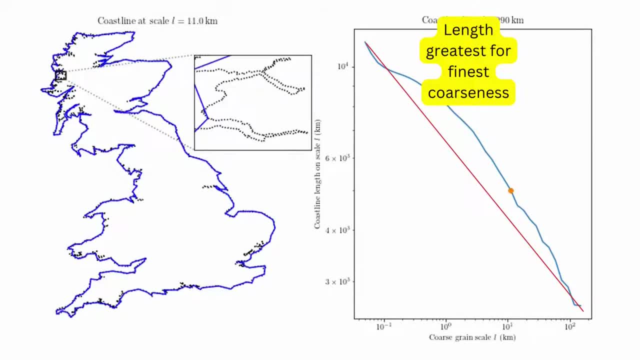 isn't actually a fractal. it just behaves approximately like a fractal for some range of scales or range of coarseness with which we're measuring it. When it comes to financial markets, we're not really interested in the length of the coastline, We're interested in the length of the. 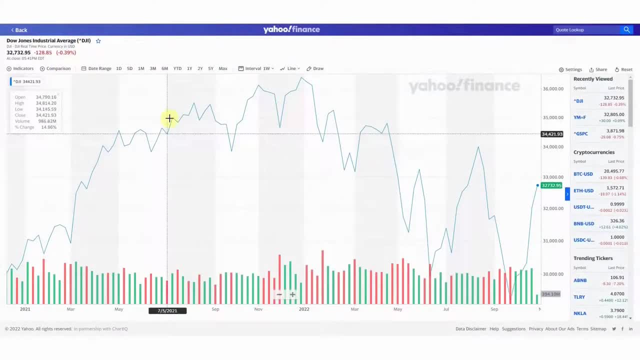 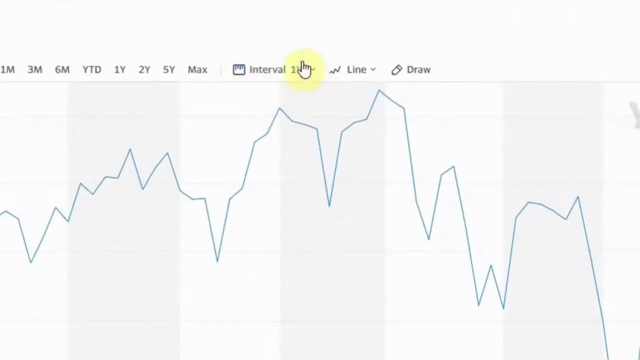 curve that describes the fluctuation in share prices or currency prices or whatever it is. But what we do have to be aware of is that if we're looking at data plotted according to some scale, say weekly data for example, then if we replotted that data on a different scale, say 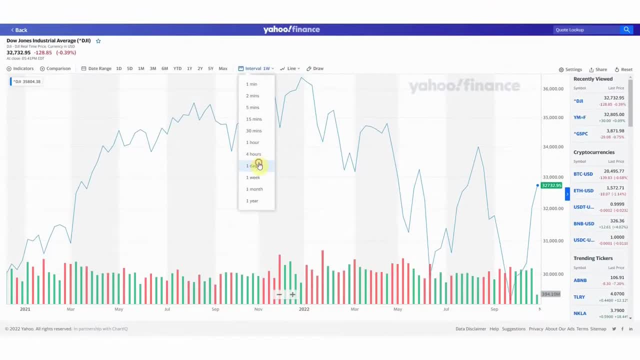 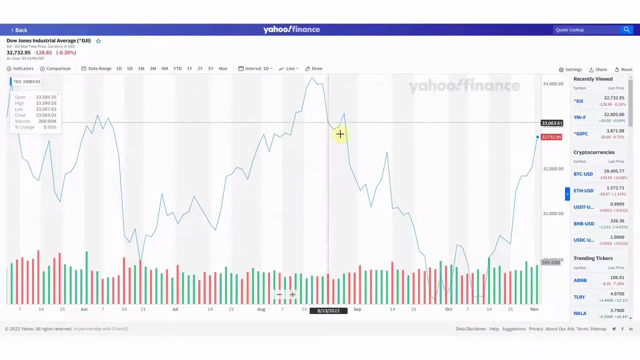 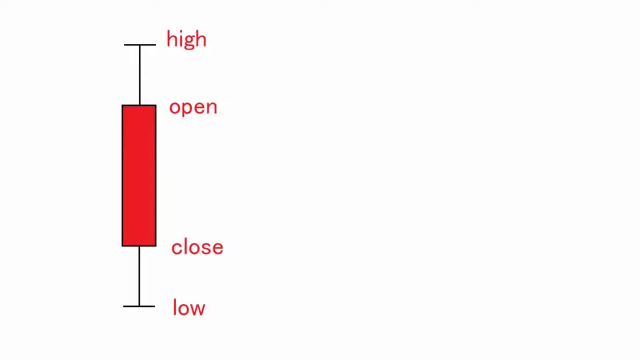 daily data. it's going to reveal a whole lot of additional information that was previously hidden, And that's really the main reason why financial market charts often use candlestick representations, which capture the daily high and the daily low and the closing price, because this helps represent some of the underlying structure and the market fluctuation. that isn't 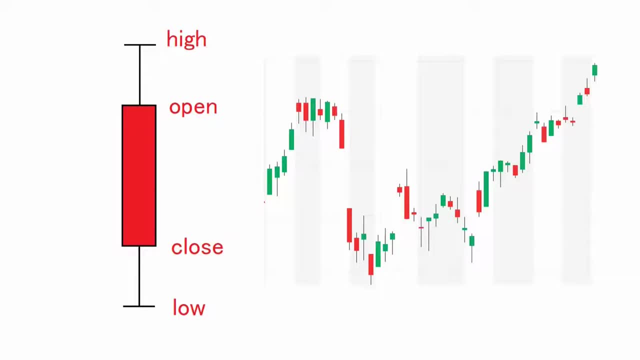 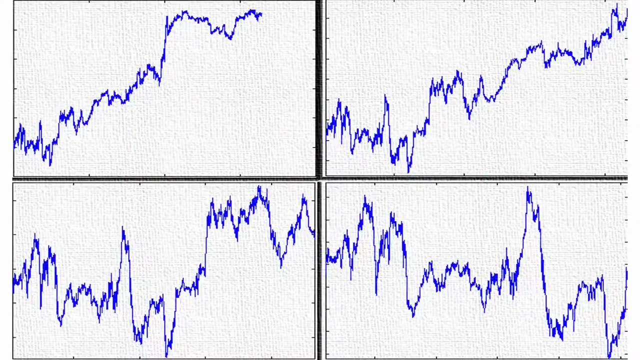 captured in a daily chart. So just to remind you that this really does apply to financial markets, we'll pull out the slide that we had previously seen in another video where we're looking at foreign exchange data and, if we look at the images or the, the market data. 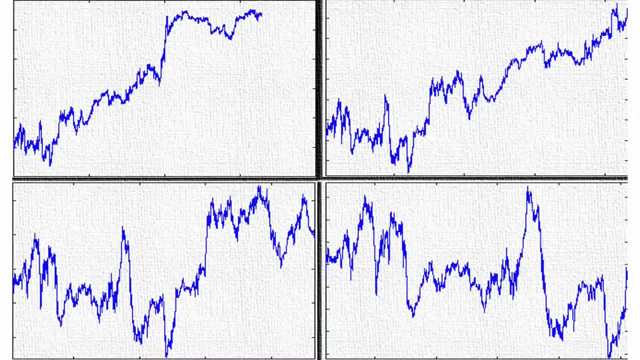 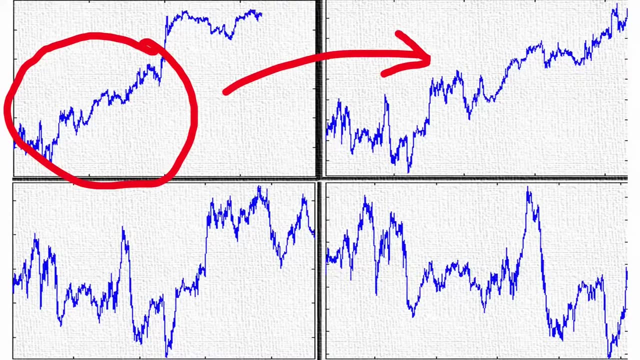 in the four quadrants of this slide we see that all this data looks like financial market data. that could easily be forex data, But the trick here is to recognize that actually all this data is literally the same data, where the data in the top right is just the same as the first half of. 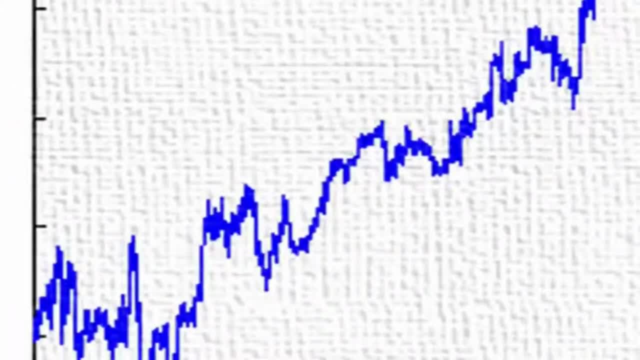 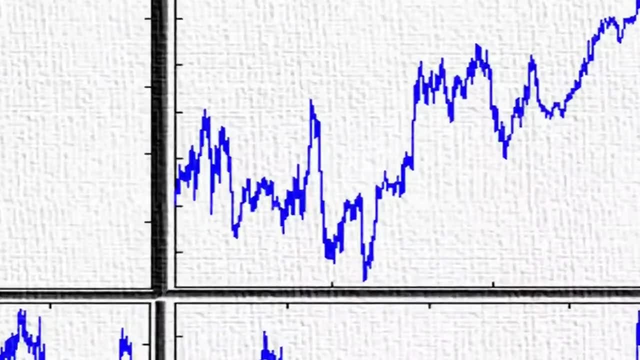 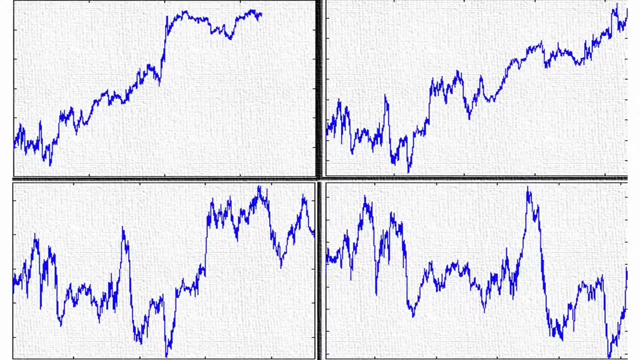 the data on the top left. so we've just zoomed in and rescaled the first half of that data, And then the data in the bottom left is the same as the data on the bottom right, data in the top right, but just the first half of that data and likewise the relationship between 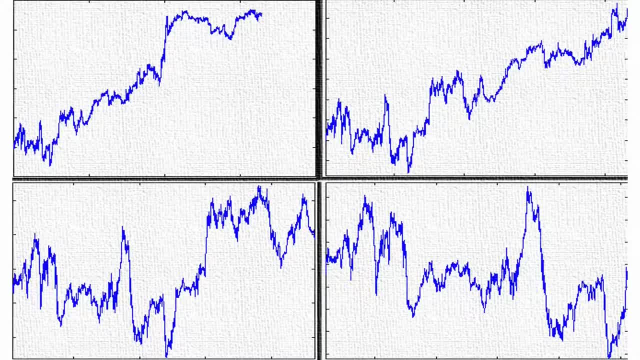 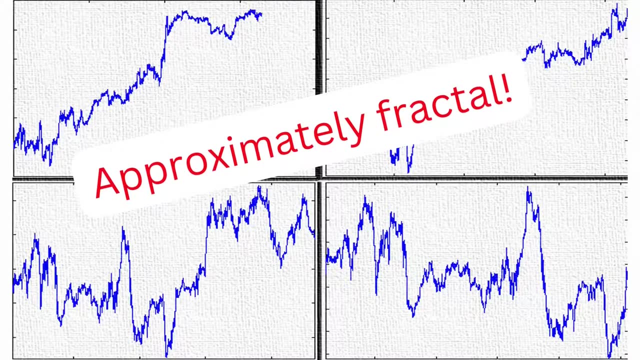 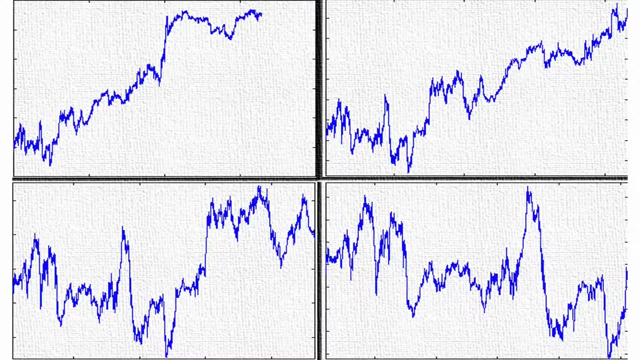 the data in the bottom left and the bottom right. so you see, it really is the case for financial market data, at least for some range of scales. and remember, just like with the british coast, financial market data is only approximately fractal for some range of scales. we see this behavior that zooming in on smaller and smaller bits of the data ends up generating. 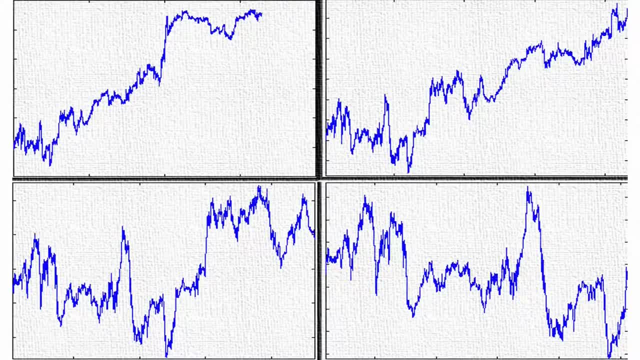 a picture which is almost indistinguishable from the larger scale. ie, you wouldn't have necessarily have just guessed that all these pictures are just zooming in on a single set of data, unless, of course, you'd seen this previous video. but then that's cheating, isn't it though? 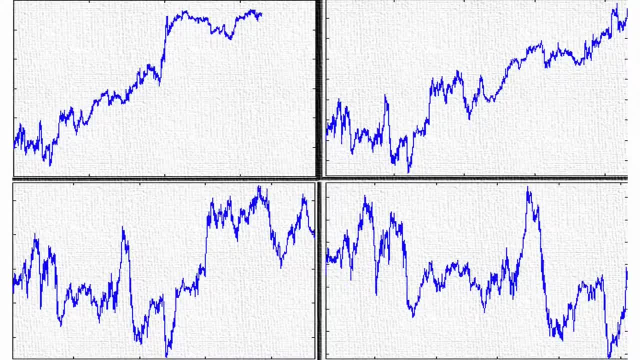 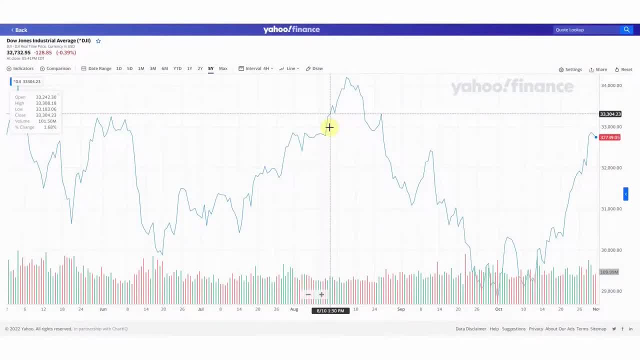 i'm cheating a bit here by reusing it, but we can demonstrate this as well by using yahoo finances plotting capabilities. so if i look at this chart of the dow and i go ahead and i click on different time periods for this and then i go and rescale this chart, you can see. 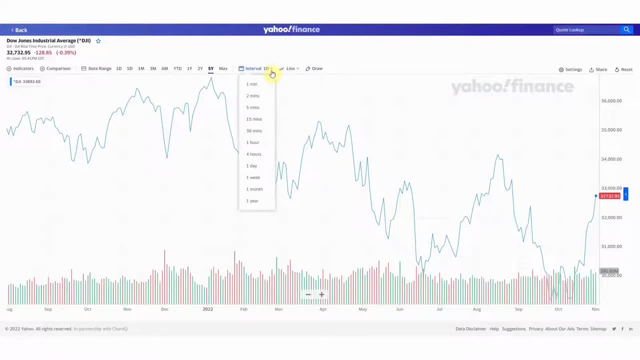 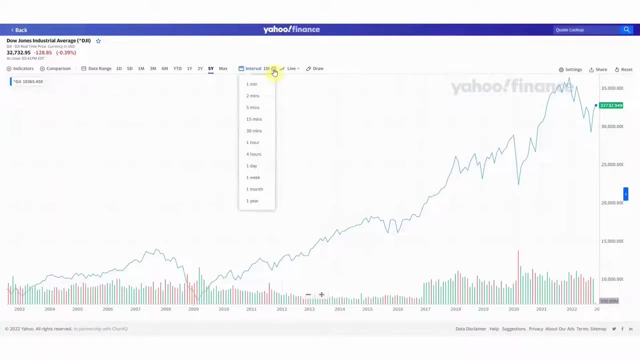 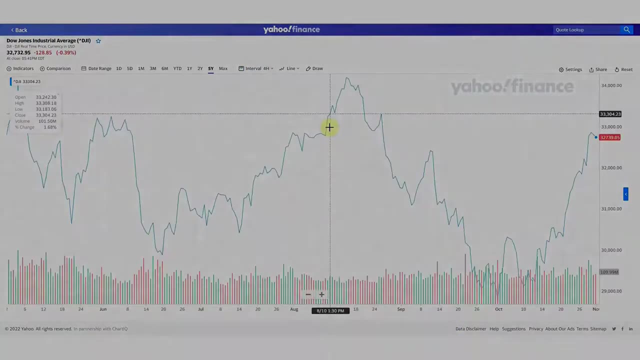 that for the time scales i'm looking at here. there is a great deal of similarity in how the charts look regardless of the time scale i'm choosing, but the couple of additional extra point that i refer to as being really important earlier on are that this scaling property also describes the hierarchy. 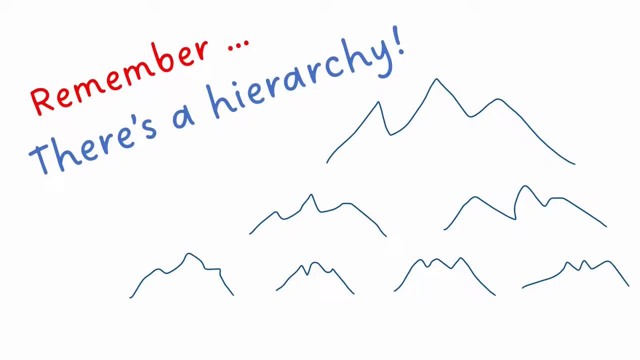 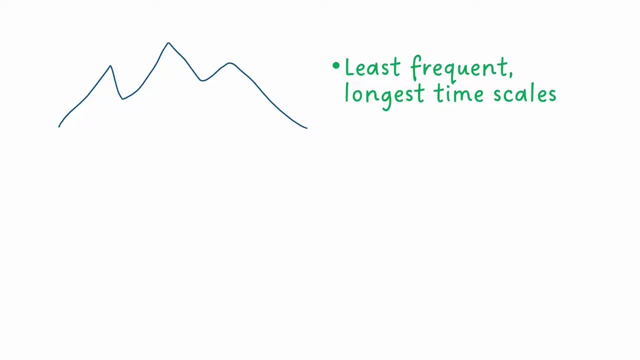 with which we see different sized fluctuations of different durations, and what we find is that larger fluctuations in the price of a stock or currency or commodity tend to also be associated with longer time scales, but they are also less frequent, and this type of is referred to as a power law and, put very simply, what that means is that big fluctuations are. 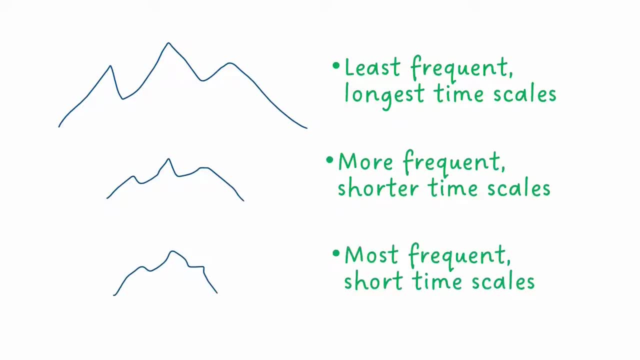 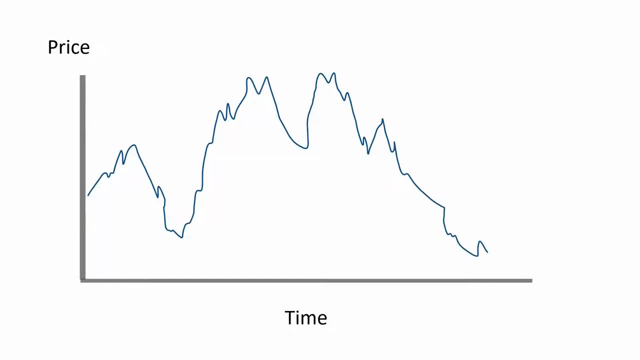 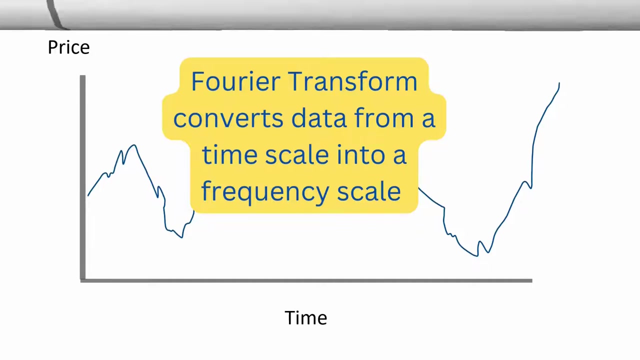 quite rare. more medium-sized fluctuations are a bit more common and small fluctuations are the most common now. if we take a time series of financial market data and do a four-year transform of that, we can generate what is called a power spectrum for that data, and it's going to. 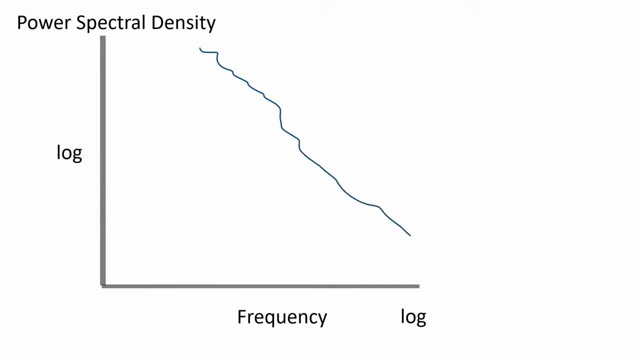 look like this, once again plotting a time scale, and then we can generate a power spectrum for that data, and it's going to look like this on a log, log scale. the y-axis here is the power energy, or however you want to think about this- involved in a particular fluctuation. so in the context of a financial market, we're probably 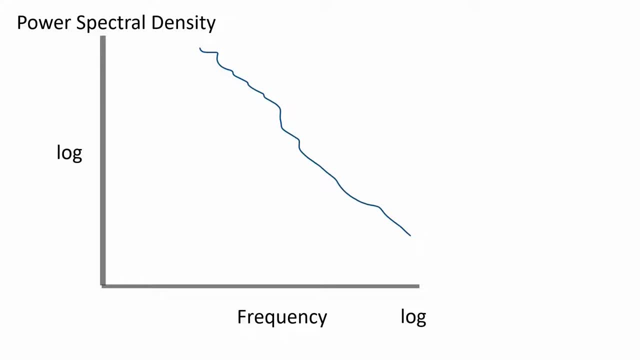 talking about changes in market valuation of a stock rather than literally, energy or power. and since the x-axis is the frequency, the left-hand side reflects events which have the longest periods. again, the biggest fluctuations have the longest periods and going to the right, this follows an approximately straight line and what we see is that the highest frequency fluctuations 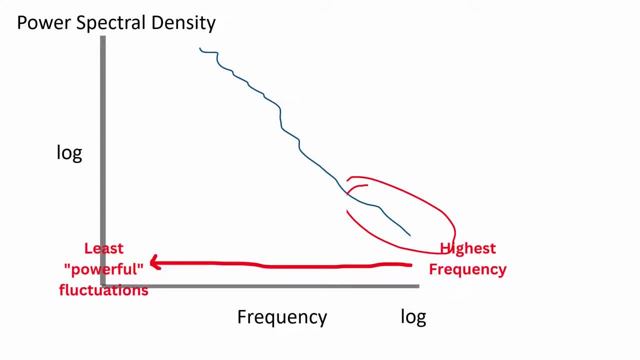 involve the least change in price. now, going back to the left-hand side, this relationship doesn't continue indefinitely. the part of the spectrum furthest to the left can be thought of is the energy containing range, and this is what's ultimately driving the most of the fluctuation in the commodity price. these reflect long-term changes in the 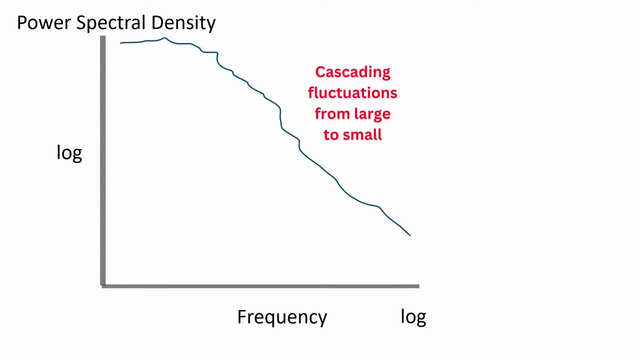 value of the commodity, whereas this middle straight line section is all about the hierarchy of the fluctuations that occur, which are more about the market price fluctuating as investors try to estimate the impact of those longer-term fluctuations. so in every large movement in a price of a commodity, 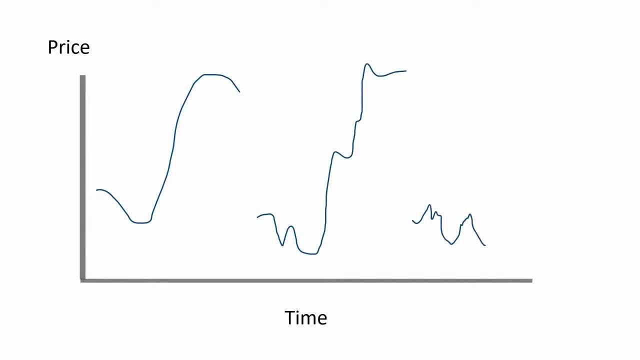 or a stock. there will be multiple movements sitting on top of that, and on top of each of those there will be smaller fluctuations again, and this is the process by which large scale fluctuations end up getting passed down to smaller and smaller scales. now, if you're wondering where all this terminology comes from, 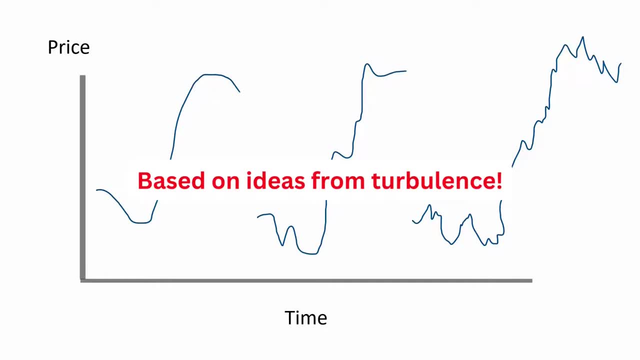 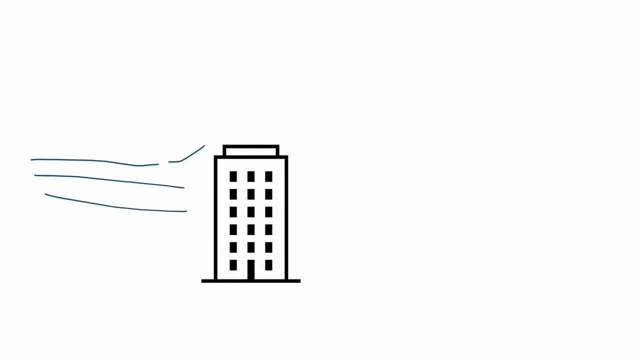 funnily enough, it comes from the study of turbulence. so in turbulence we might have strong winds hitting some kind of object around which the wind curves. this generates eddies, and eddies generate from them smaller and smaller eddies which pass down their energy from. 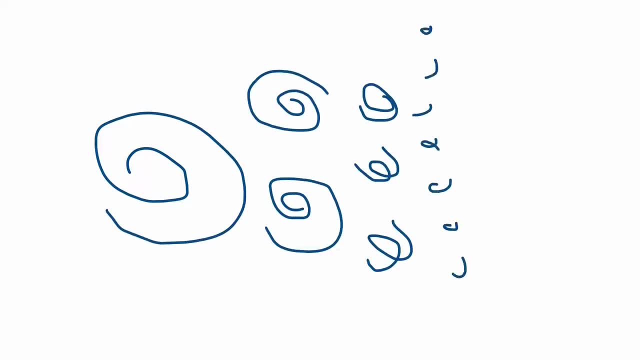 the large scale to the small scale almost losslessly, and that's reflected in the straight line part of the curve here. this is what's called the inertial sub-range of turbulence. it's where all the eddies occur and the hierarchy of eddies, and it's really quite a peculiar thing. 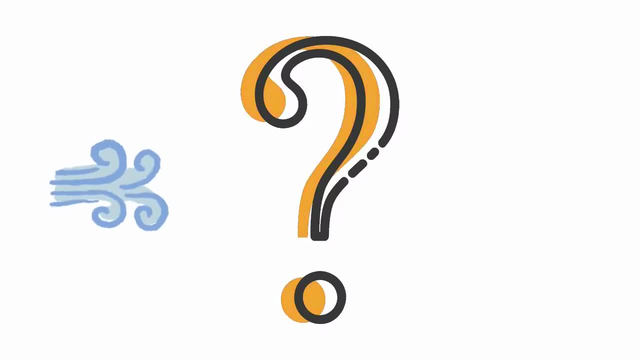 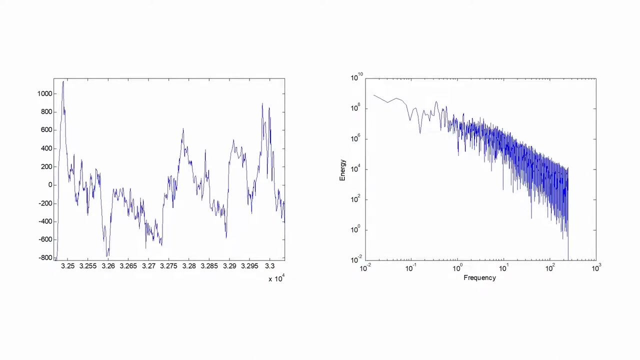 that the behavior of turbulence, which really has not very much to do with financial markets at all, of well, nothing really should have so many statistical properties like this in common with financial markets. in fact, if i were to show you a chart of turbulent data, it would be easy for. 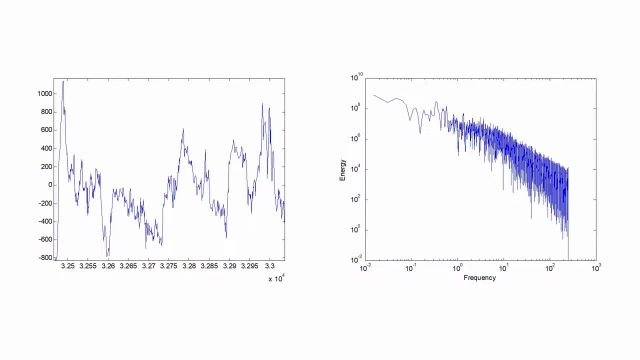 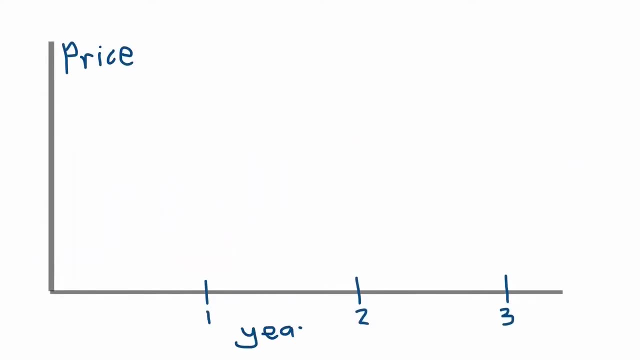 you to mistake it as a financial market chart, and here's one here just to prove that point. the final point to note here is that the dynamics over the long term don't sit in this inertial range. therefore, they're being driven by longer-term fluctuations and the underlying strength of a stock or an economy and when. 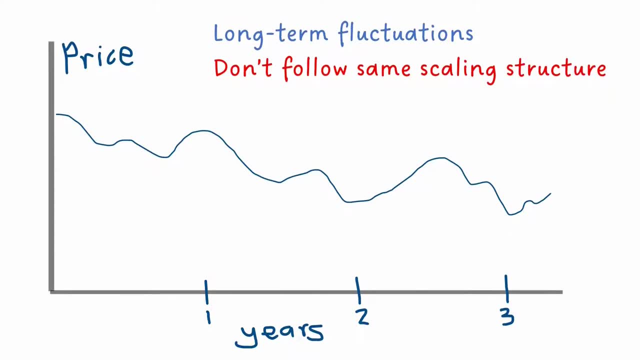 looked at at this scale, the data doesn't have these fractal scaling properties, so there is a particular range, and it's perhaps over the period of a year or two where the fractal nature of financial markets no longer really applies. another interesting thing about that is that this sort of implies that this shorter term fluctuations 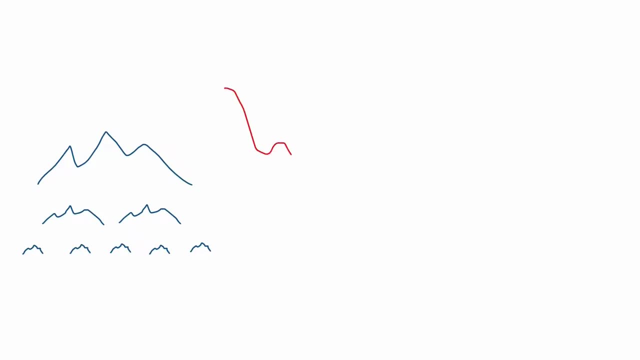 don't necessarily represent changes in the underlying fundamental value of the stock or currency you are looking at, because they exist, because these fluctuations must obey this hierarchy, but the hierarchy has nothing to do with the underlying value of the stock, except where it makes a difference to the underlying value in the long term, which